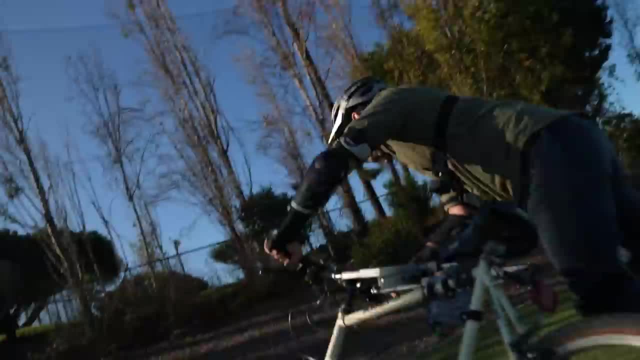 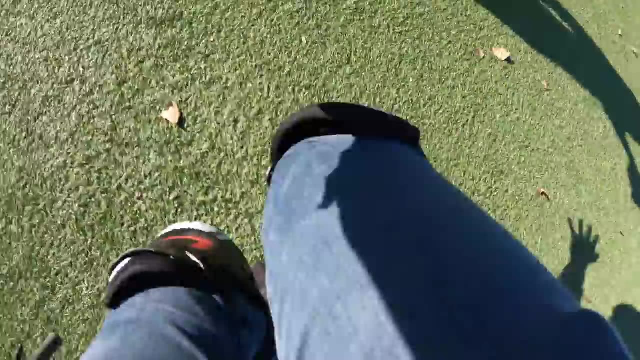 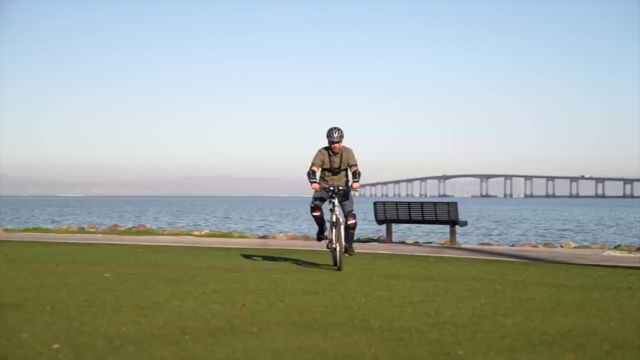 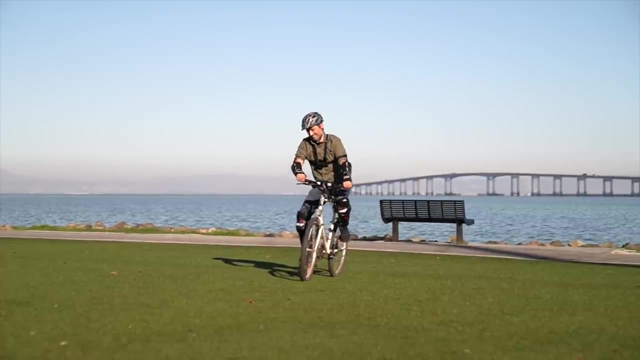 but there is no chance in hell. Left Right, All right. Left Right, right, right, God. If you look closely, you can see the problem Here. I'm trying to turn right, but steering that way puts me off balance. If you could ride this bicycle, you would find it's impossible to turn. 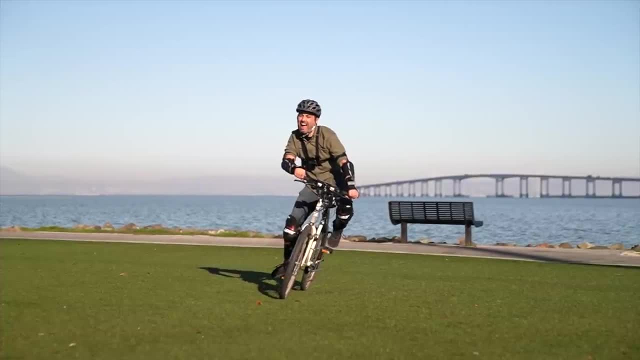 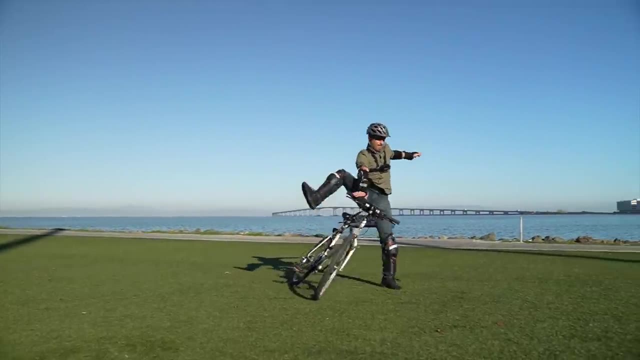 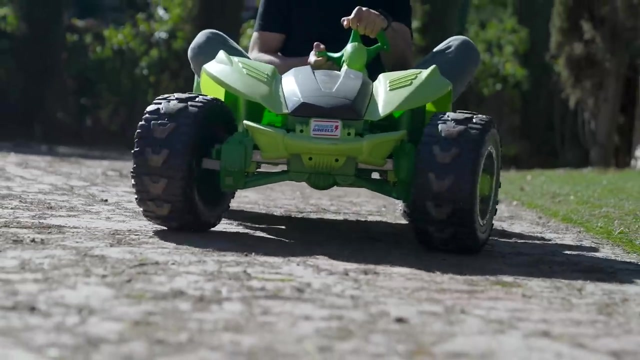 left without first steering right, And it's impossible to turn right without first steering left Right. This seems wrong. I think most people believe you turn a bike simply by pointing the handlebars in the direction you want to go. After all, this is how you drive a car: Point the front wheels. 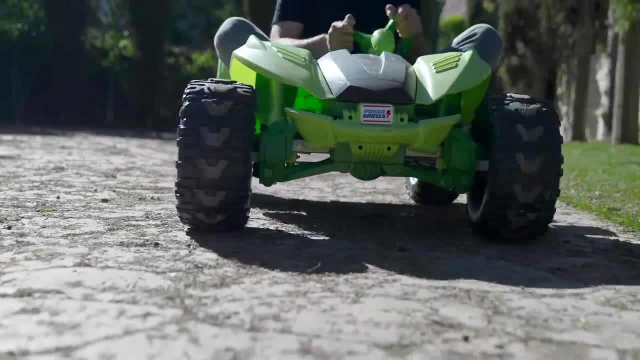 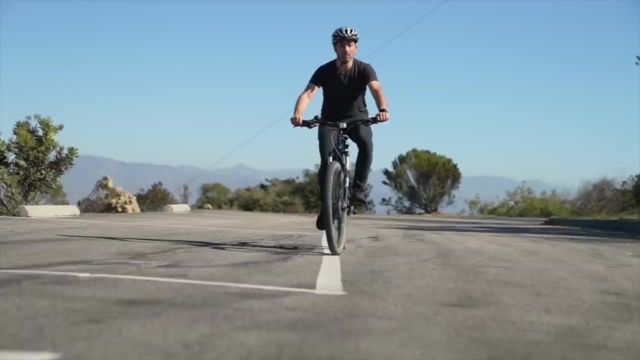 any direction you like and the car just goes that way. But the difference with a bicycle is steering doesn't just affect the direction you're headed, It also affects your balance. Imagine you want to make a right turn, So you steer the handlebars to the right. 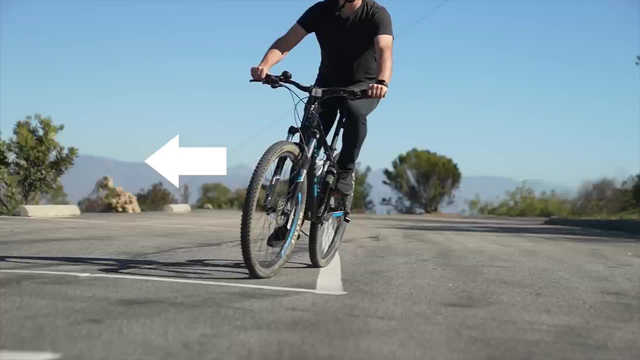 What you've done is effectively steered the bike out from under you, So now you're leaning to the left And the ground puts a force on the bike to the left. So the only way not to fall is to steer the bike to the. 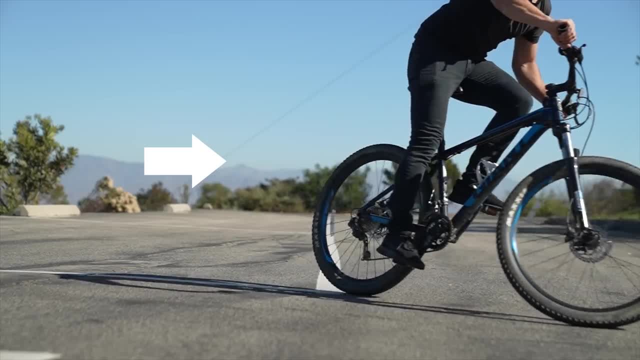 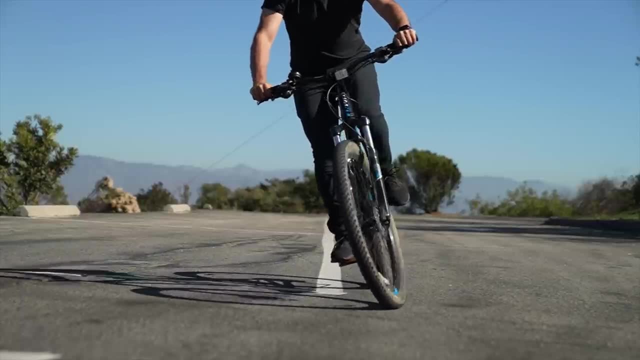 left. You have made a left turn. If you really wanted to turn right, you first have to counter steer to the left So you can lean right into the turn. This is something anyone who rides a bike knows intuitively, but not explicitly: Turn left. 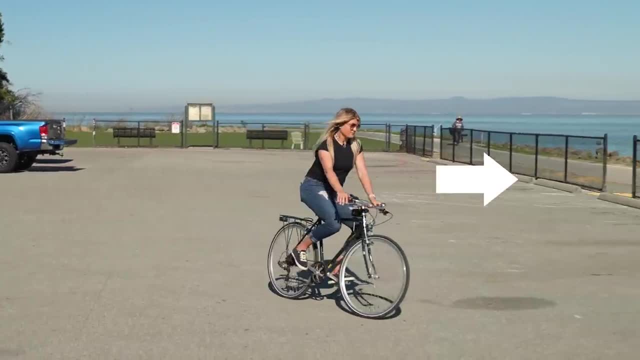 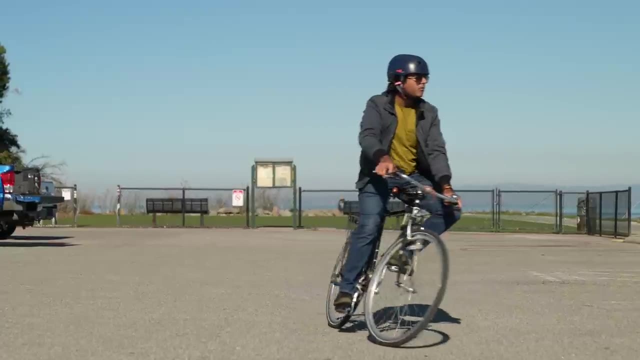 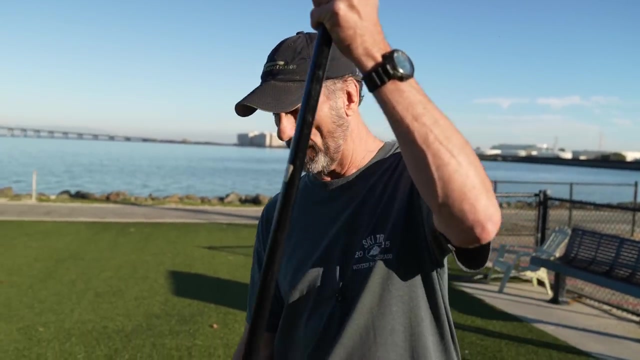 Film someone riding a bike towards you and tell them which direction to turn, and you will find that they counter steer, without even thinking about it, Hard left When you're riding a bike. it's exactly the same as what we call an inverted pendulum or balancing a broomstick on your hand. If I'm 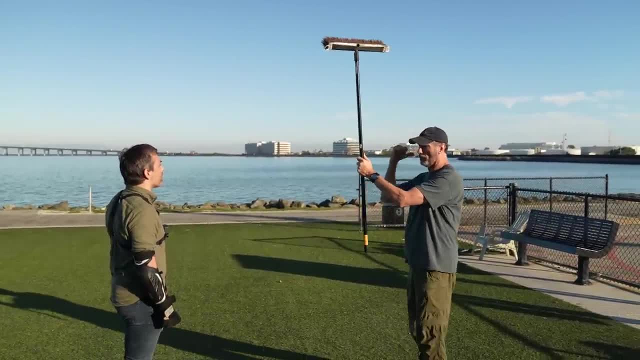 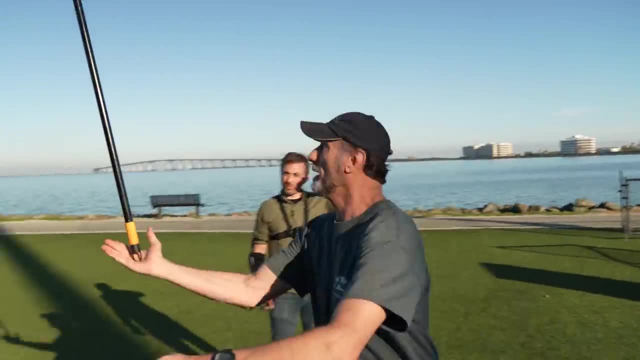 balancing it and I just start walking toward you. it will always fall away from you. If I want to walk toward you, it's easy enough to do and people inherently know how to do it. If I pull it backward, I can now start walking. that way I have. 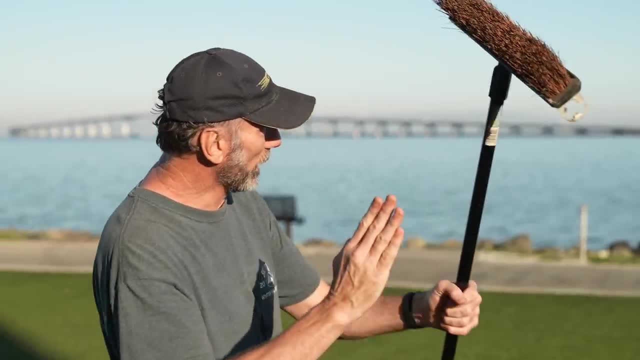 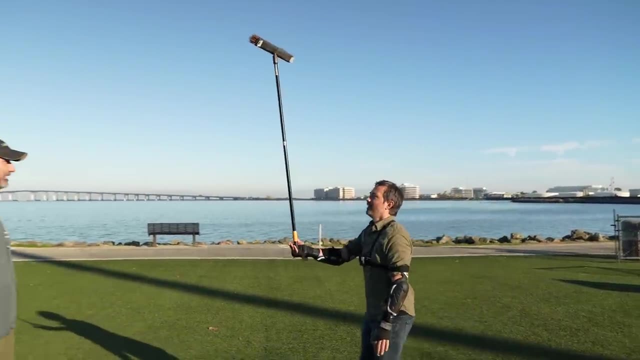 to initiate the lean, to turn into it. If you want to move the pendulum somewhere, you first move the base in the opposite direction, and now the pendulum is leaning in the direction you want to go, so you can move with it, And it's the. 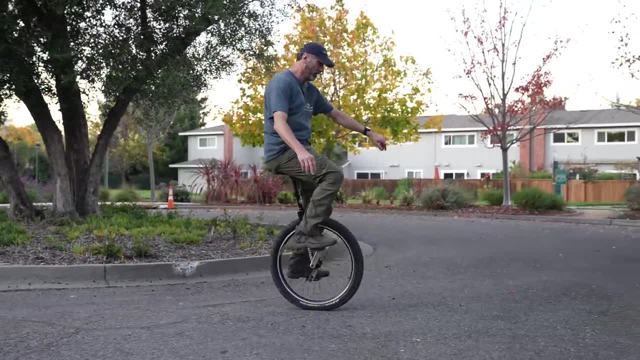 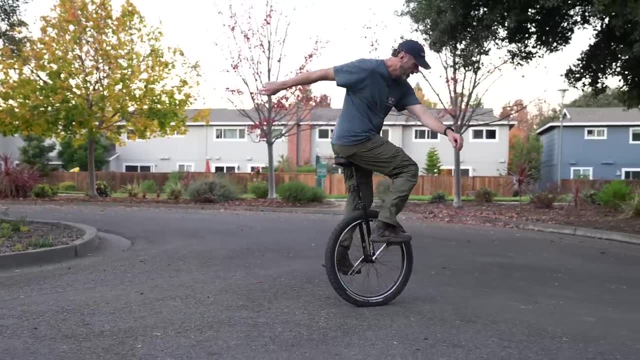 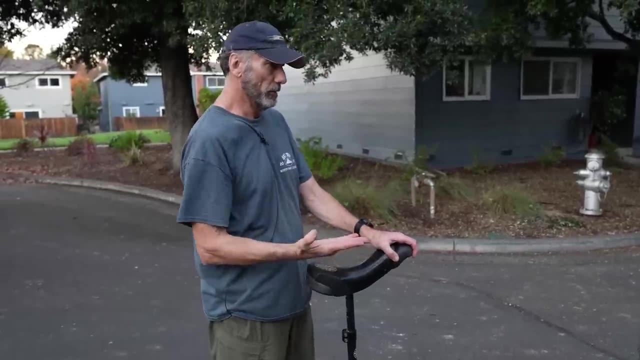 same with a unicycle: In order to go forward, first you have to pedal back, so you're leaning forward, and then you can go forward with it. Everything you're doing on a unicycle is all about keeping that contact patch right where it needs to be, relative to you. You're balancing the broomstick. It's. 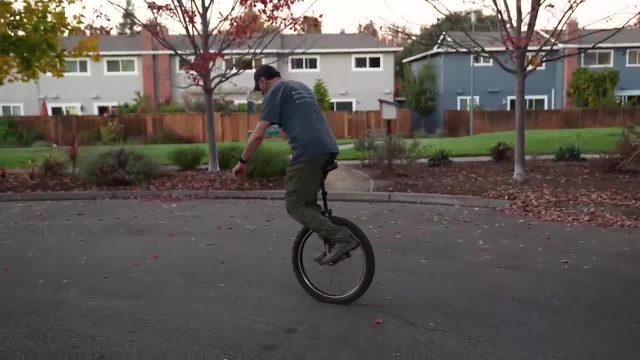 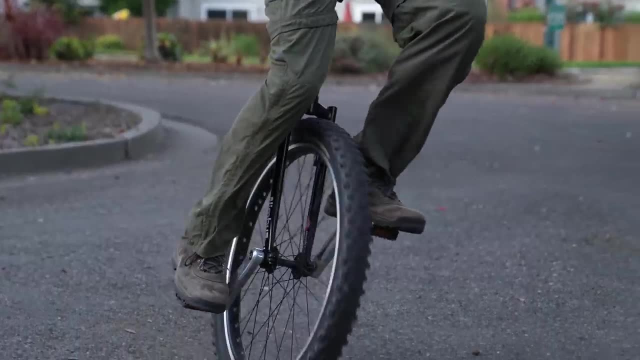 just that on a unicycle: you do the longitudinal balance with the pedals and you do the lateral balance, the side to side, the same as you do with a bike. You essentially sort of a small counter steer to get that weight, to get the contact patch out, and then you can pedal and bring it under you. Now I should. 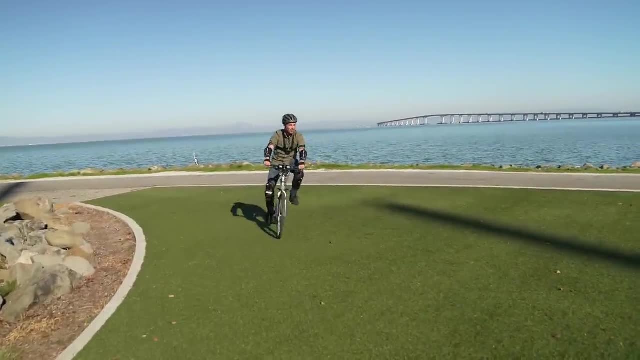 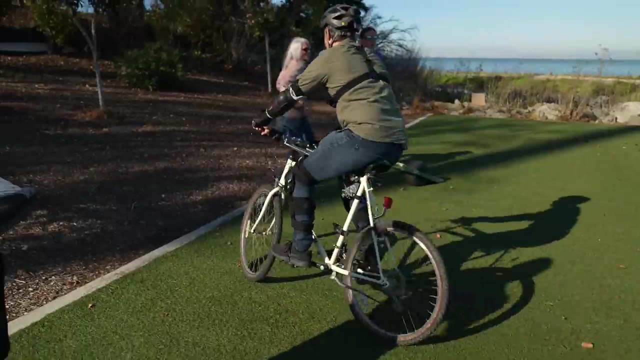 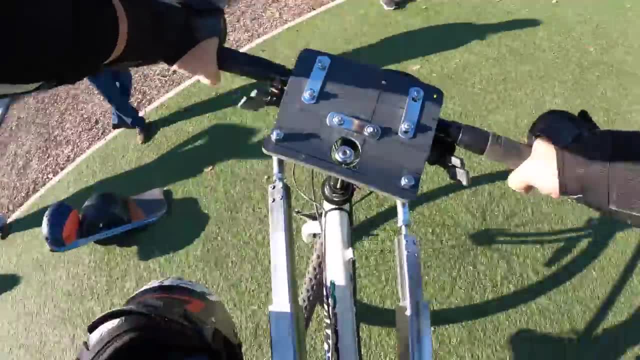 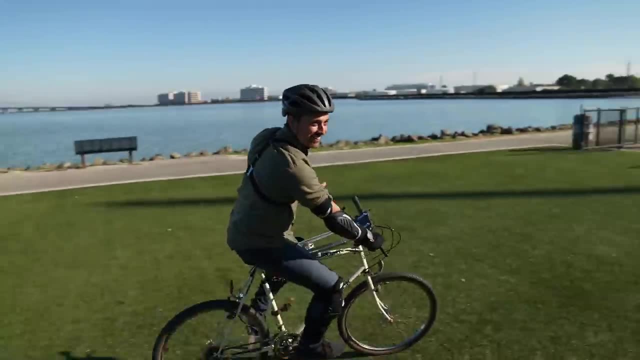 can keep going, But yeah, but don't turn left. Don't turn left, I can't turn left. What's interesting about this is it shows that you can still ride the bike perfectly well, right, It's just you can't turn left. The funny thing is that you 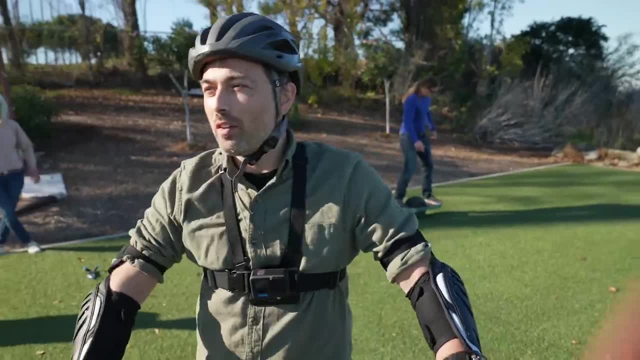 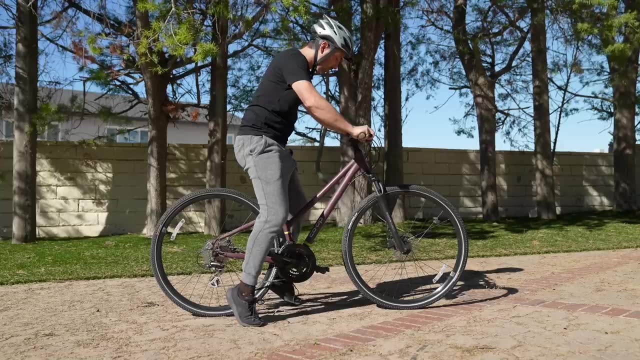 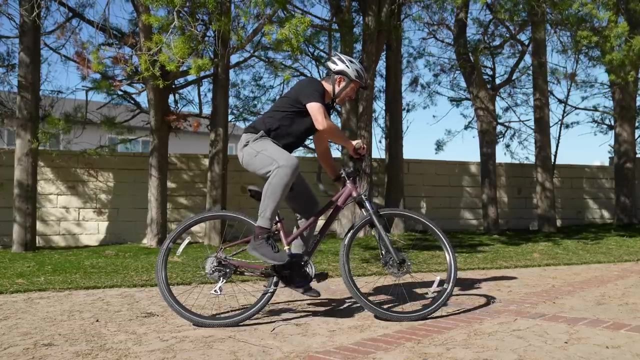 couldn't initiate the turn Right. I mean, the wild takeaway is that steering is not just for turning the bike. Steering is for balancing. That's exactly right. Why is it hard to balance on a stationary bike? I think most people believe it's because the wheels aren't spinning, so there's no. 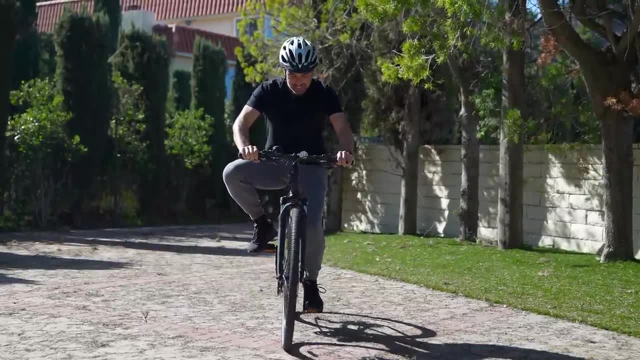 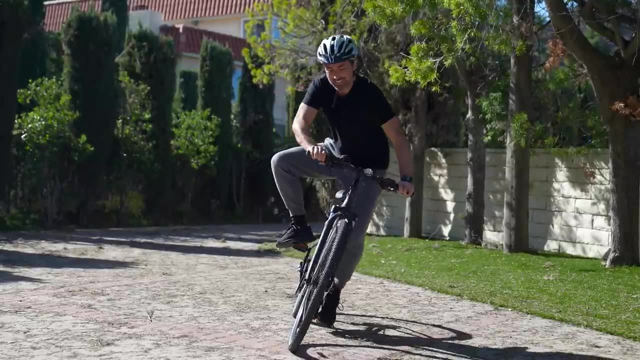 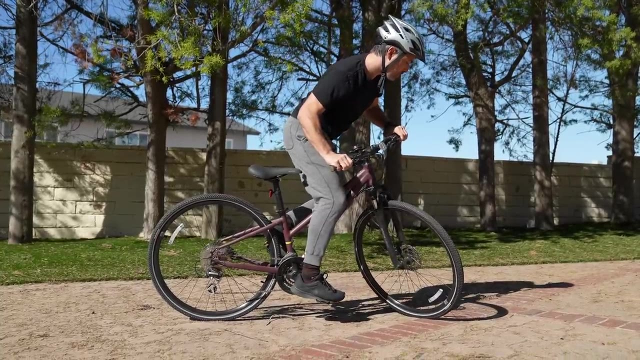 gyroscopic effect, But that's not it. The truth is, you use steering to keep the bike underneath you, But steering doesn't work when you're stationary. Your balance comes not so much from how you position your body over the bike, but by how you keep it underneath you. Even when going straight, you're constantly. 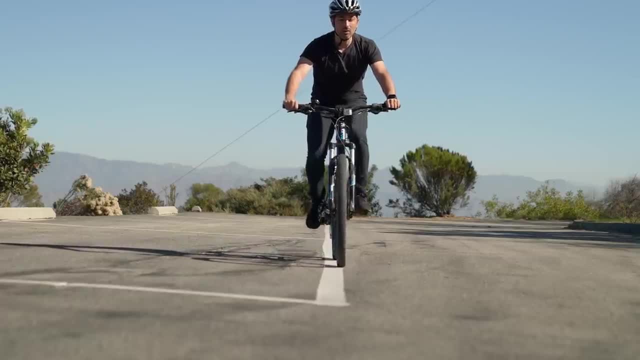 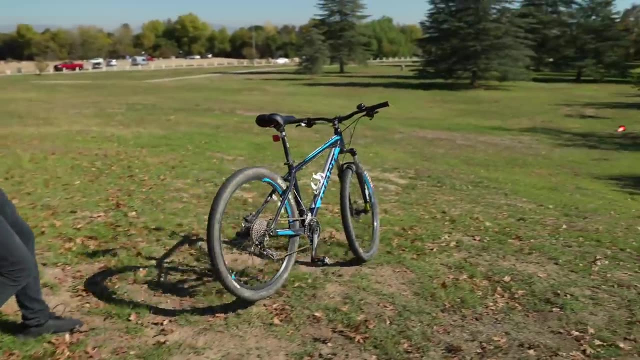 making small steering adjustments to maintain balance, You're moving the contact patch of the front wheel under you. You're doing exactly what you do when you balance a broomstick on your hand. So if the rider is responsible for steering the bike to keep it balanced, how do bikes without riders stay upright? 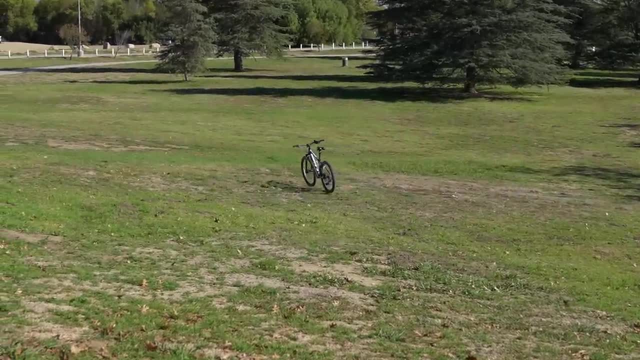 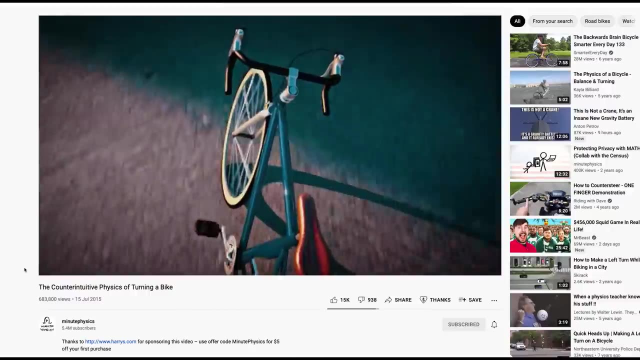 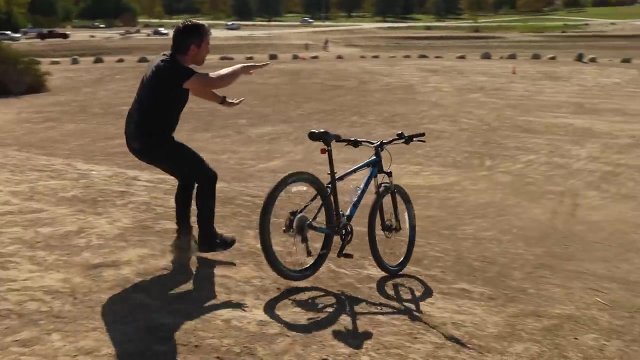 As long as a bike is moving with sufficient speed, it can keep coasting indefinitely. I first became aware of this phenomenon through the great videos on this channel. You should definitely check them out, But it turned out. the ground where we went to test this effect was really bumpy, But the bike still manages. 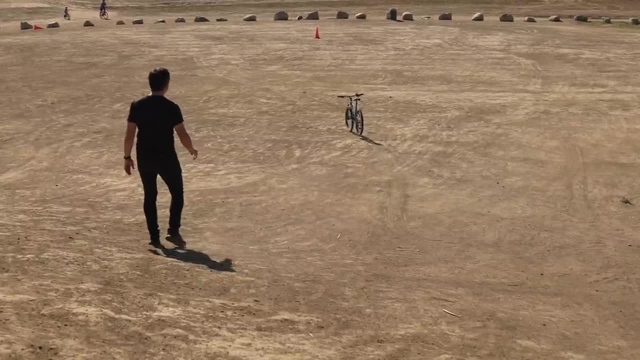 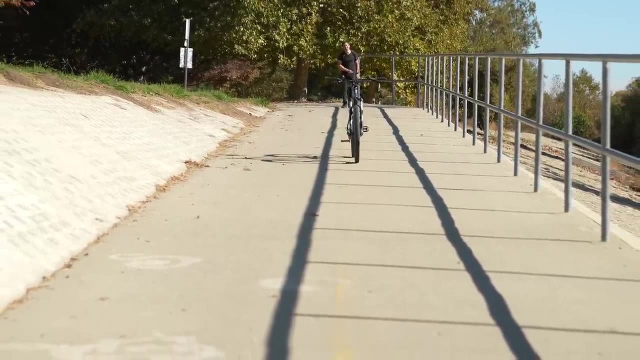 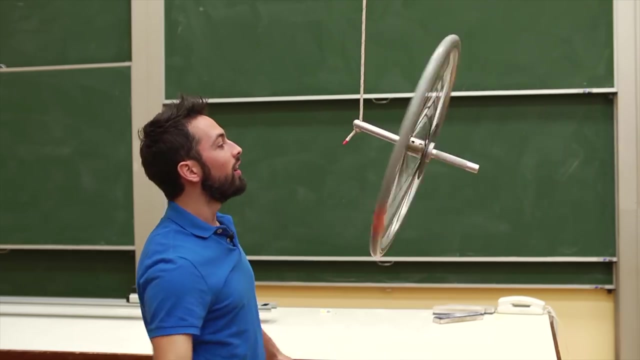 to absorb all these perturbations and remains stable. So how does it do this? I think most people believe it's the wheels spinning that creates some sort of gyroscopic effect that resists falling over, Just like in this demonstration of gyroscopic precession. the wheel stays upright even though 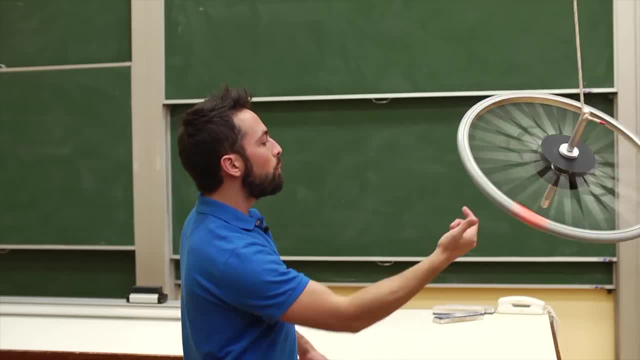 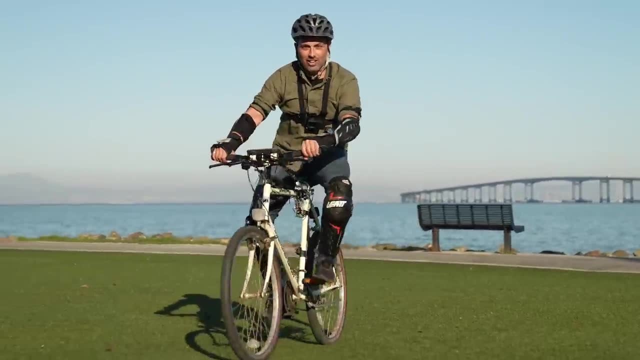 the bike is pulling it down, But this is not why bikes are stable. Just watch what happens when we lock the handlebars completely, So you can only go straight ahead. Locked out, locked out, whoa. All that's happening is the steering is locked. You just. 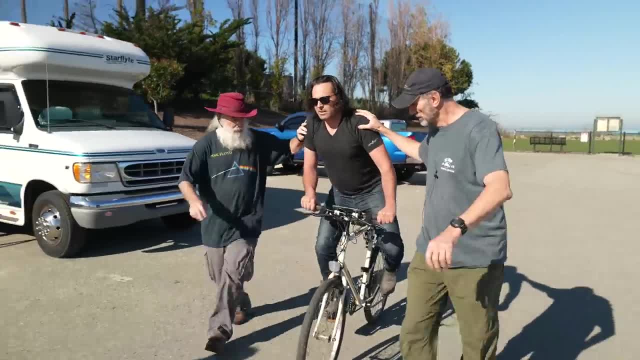 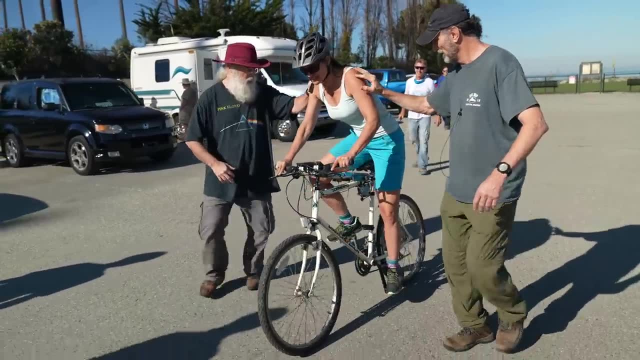 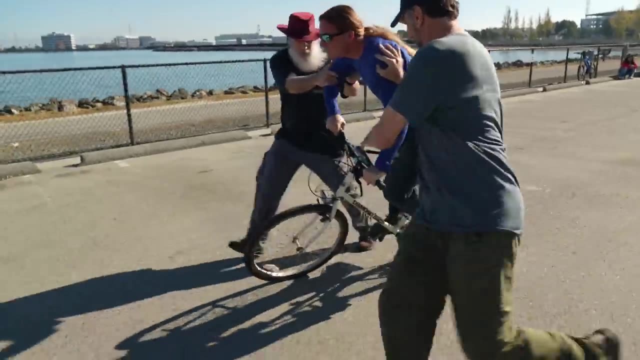 got to ride it. You don't have to turn, You just go straight, Ride, Letting go. Some people tried going really fast. Holy crap, this is impossible. Others experimented with extreme balancing techniques, But even with the gyroscopic effect of the 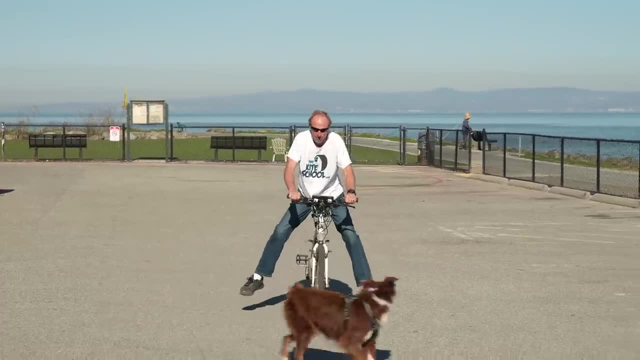 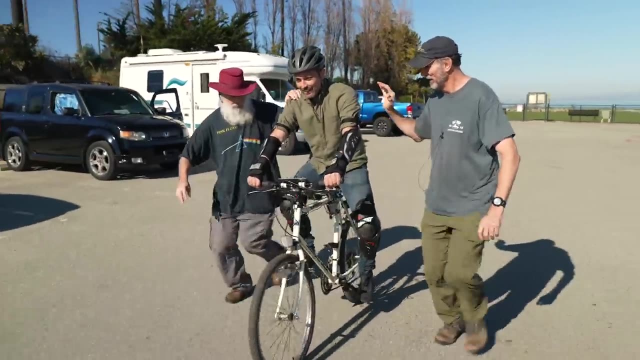 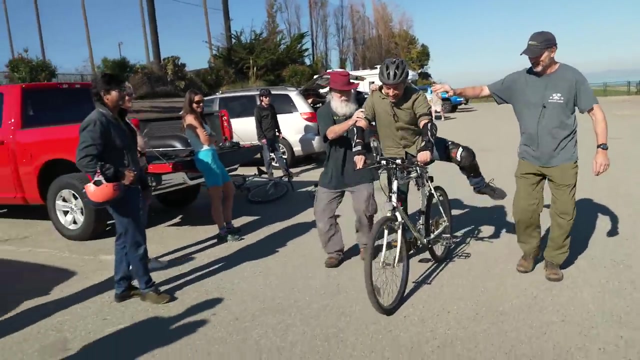 wheels. no one was able to keep the bike upright for more than a few seconds. This is not safe for a second. It is just as hard to balance on a bike with locked steering as it is to balance on a stationary bike. No, this one is impossible Because you can't steer the bike. 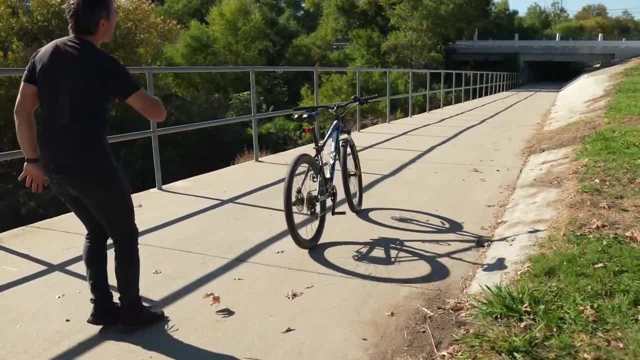 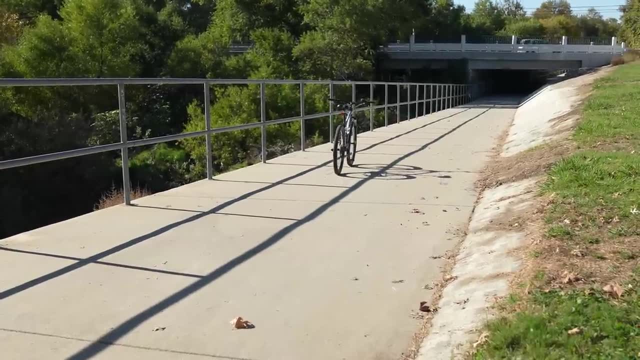 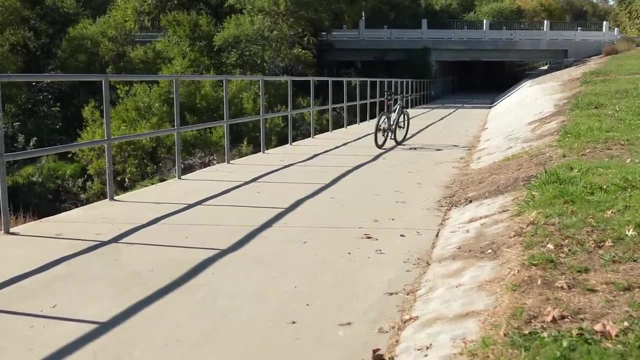 under you. The real reason bicycles are stable without riders is because they are cleverly designed to steer themselves. If they start falling to one side, the handlebars turn in that direction to steer the wheel back underneath them. At least three mechanisms are responsible. 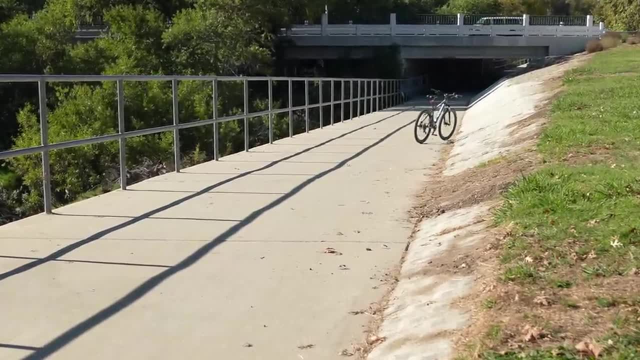 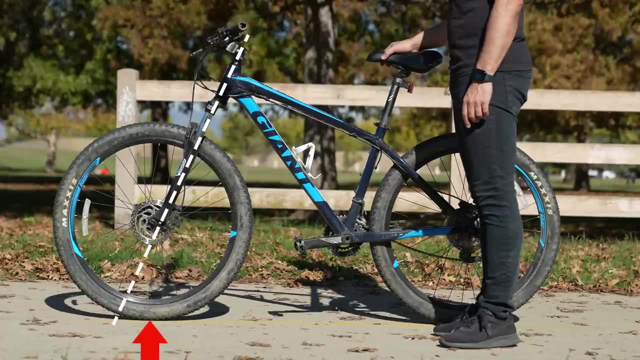 for a bikes corrective steering. The first is that, due to the angle of the front fork, the steering axis intersects the ground in front of where the wheel touches the ground. If the bike starts Leaning to the left, the force from the ground on the tire turns the wheel to the left. 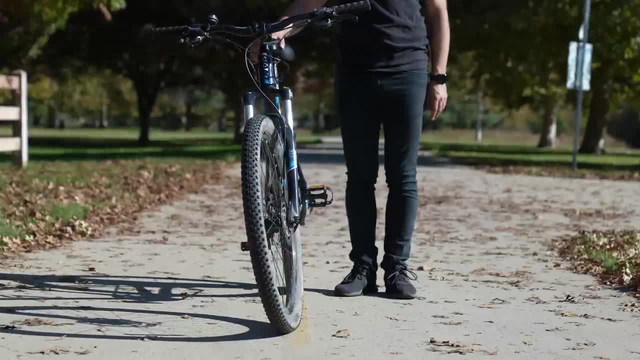 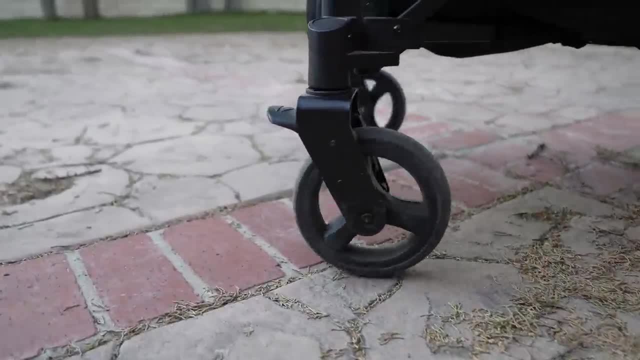 If the bike starts leaning right, the force from the ground pushes the wheel to the right. The front wheel of a bicycle is essentially a caster wheel, like those you find on strollers or shopping carts. Whichever way you drive them, the wheel falls in line and rolls in the same direction. 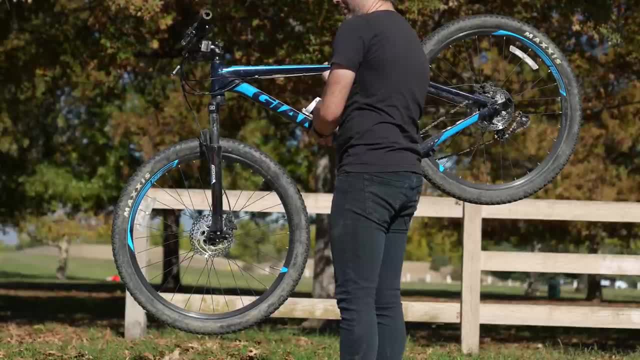 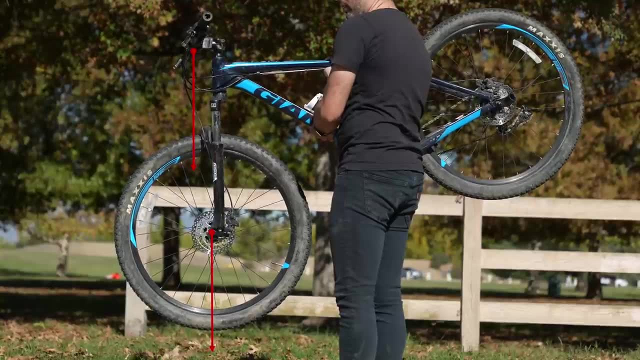 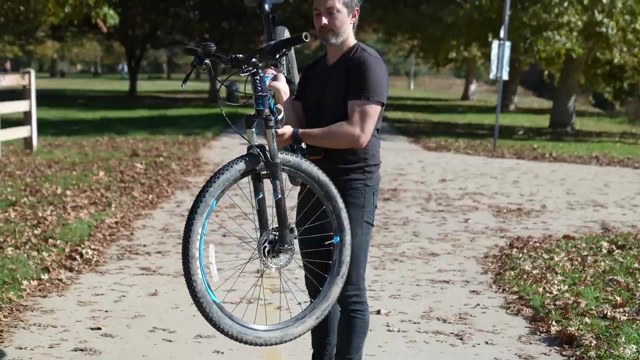 The second reason for a bike's corrective steering is that the center of mass of the handlebars and front wheel are located slightly in front of the steering axis. So when the bike leans left, their weight pushes the front wheel to the left. If the bike leans right, their weight steers to the right. 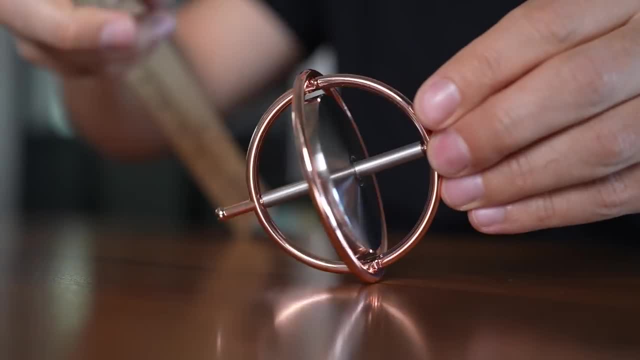 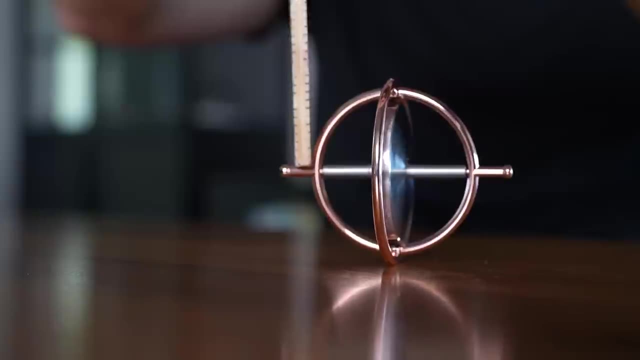 And the third mechanism is a gyroscopic effect, but it doesn't keep the bike upright directly, it just helps steer. If you have a gyroscope and you push down on the left hand side, the gyro will turn left. If you push down on the right side, it will turn right. 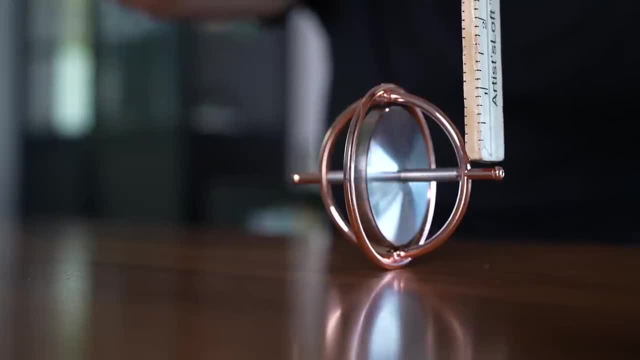 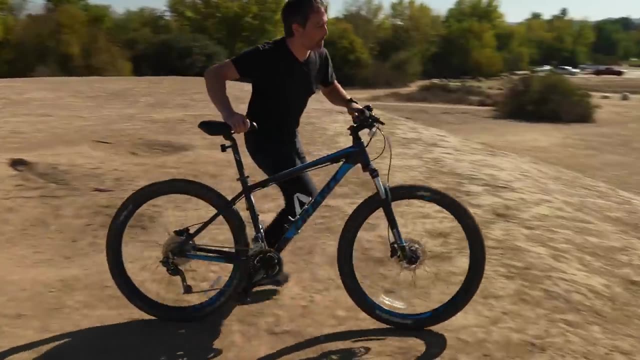 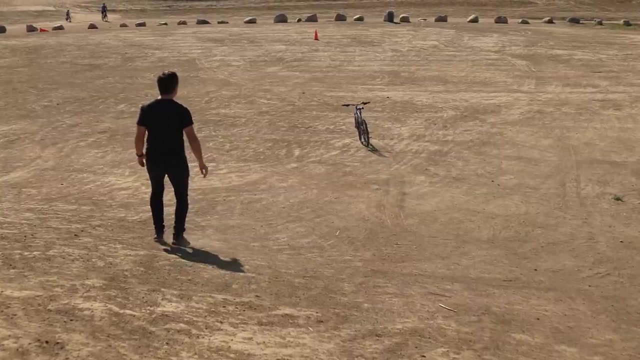 This is known as gyroscopic precession. It seems as though the force you apply takes effect 90 degrees from where you applied it. So bikes are stable primarily because of steering. They have built-in mechanisms for steering themselves. In fact, you don't need all three mechanisms to create a stable bike. 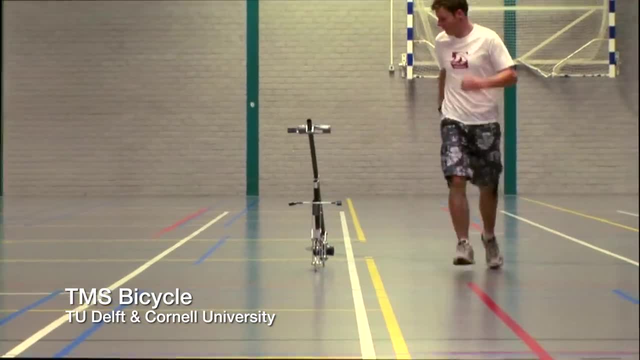 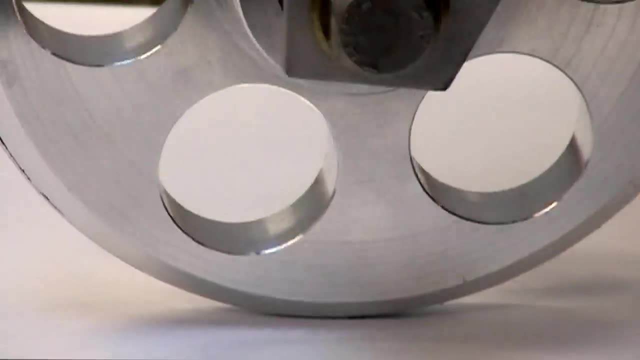 Researchers created this weird-looking bicycle to prove a point. It has no gyroscopic effect thanks to counter-rotating wheels above the wheels that touch the ground. Plus, there is no caster effect because the front wheel touches the floor in front of the steering axis. 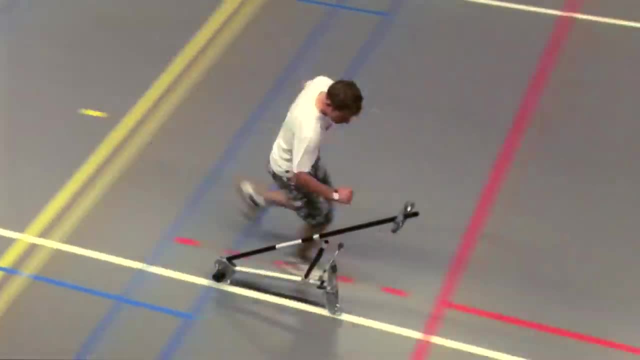 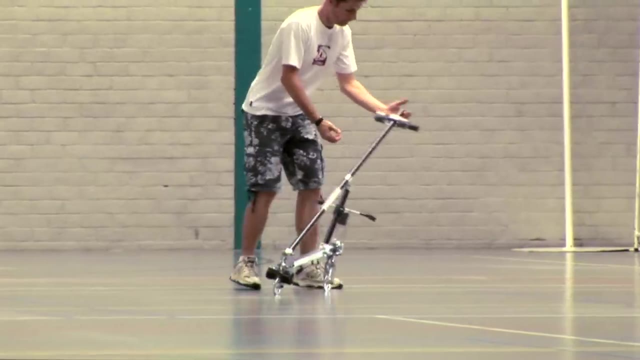 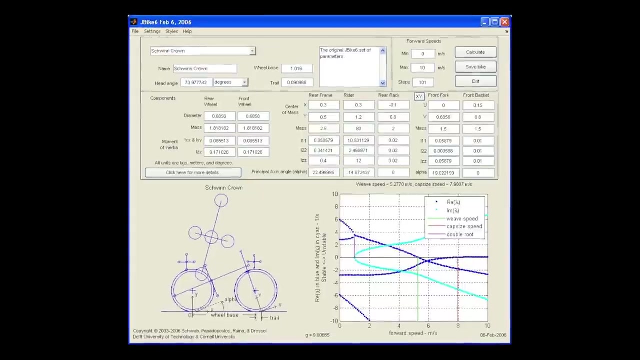 But this bike is made stable by its mass distribution, the force of gravity on which steers it in the direction of any lean. Understanding how bicycles work is still an active area of research. There is a program you can use to input all the different bicycle parameters and see the 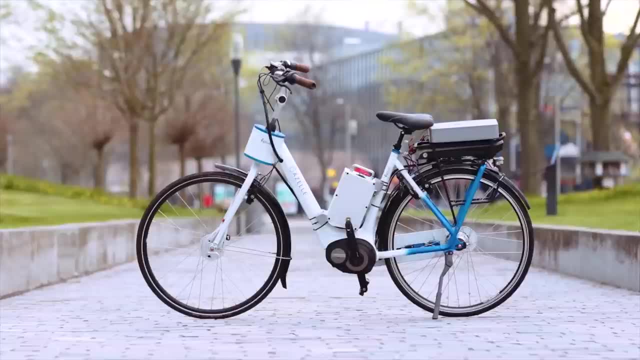 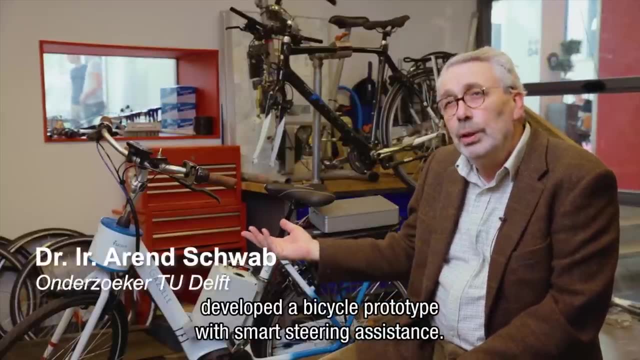 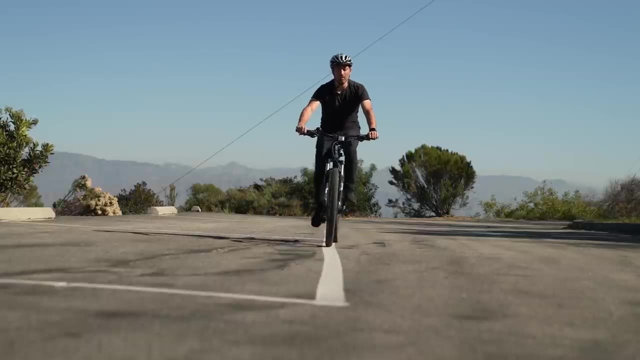 range of speeds over which it is self-stable, And this research is leading to better bikes. This prototype has a smart motor in the handlebars to actively help steer, keeping the bike upright even at low speeds. I guess it's fitting that we're still learning new things about bicycles, since most of us 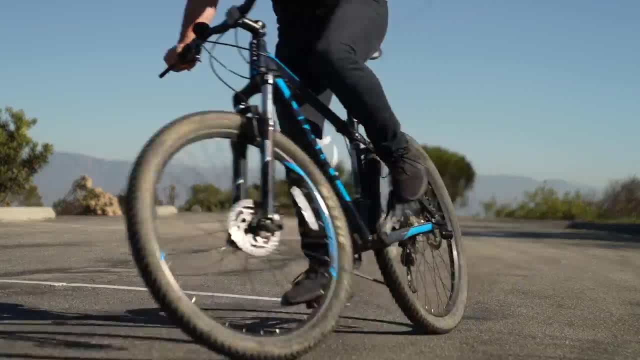 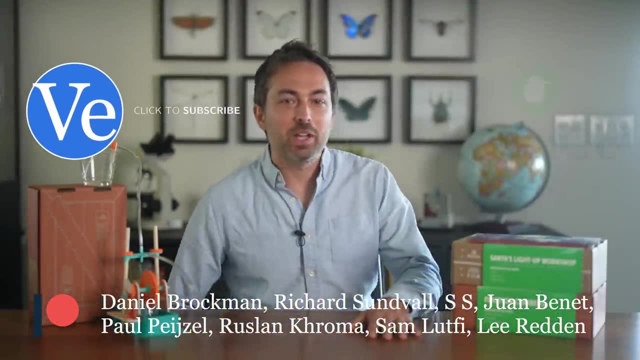 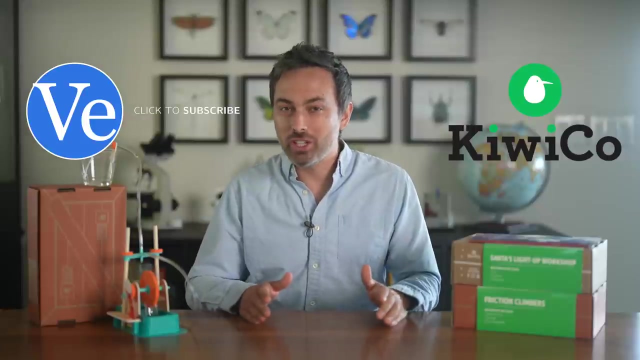 are able to ride one without any knowledge of how we're actually doing it. Hey, this video was sponsored by KiwiCo, creator of awesome hands-on projects and toys designed to expose kids to STEAM concepts. With the holidays fast approaching, a KiwiCo subscription is the perfect gift for any of 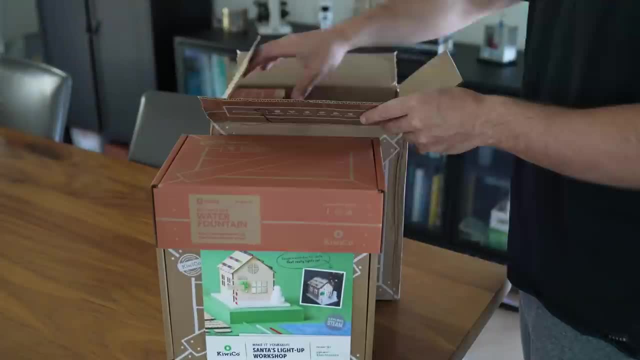 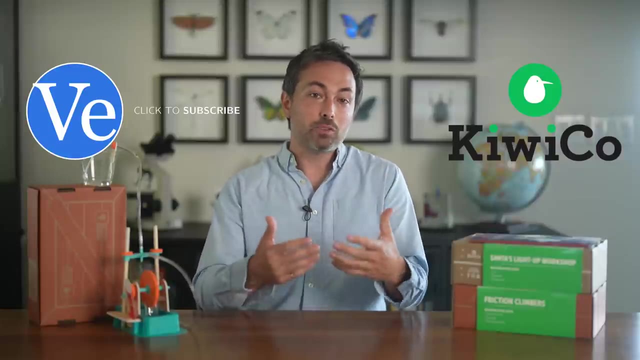 the young people in your life. KiwiCo now has 9 different subscription lines for different age groups and topics. Plus they ship to more than 40 countries. I think it's such a great gift because each month, a box turns up at your door and provides.